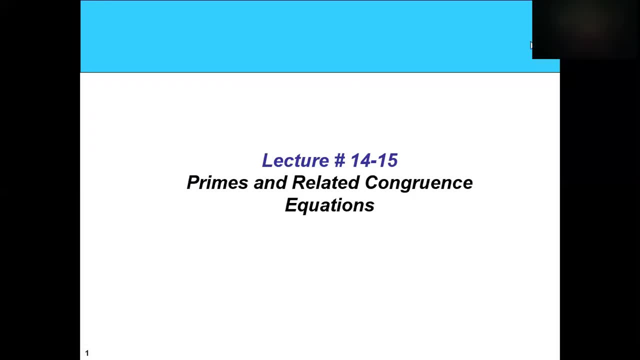 Dear student, I hope you are fine and doing well. Today our lecture is about prime and related congruence equations. It is basically the continuation of our last lecture. Basically, our last two lectures were related with the number theoretic basic fundamentals that are: 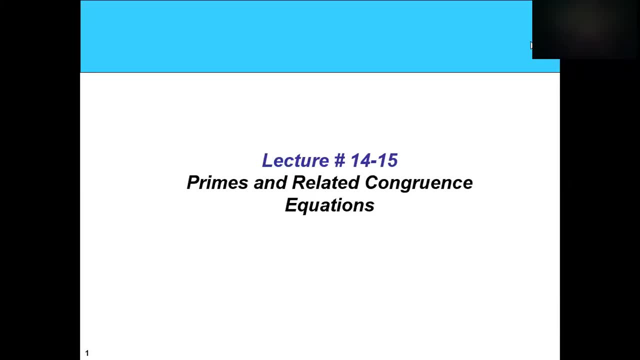 required in public key cryptography. So these are again our two lectures that are fundamentally based on number theory, and these definitions are required in public key cryptography. So let me introduce you to the second lecture, something that is prime related: common class equations and and some other ideas. 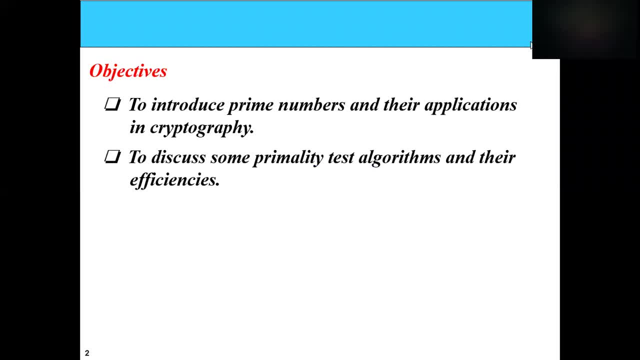 let us start today lecture. the objective for today lecture is to introduce prime numbers and their cardinality and their importance in cryptography. moreover, we will discuss some primary tests, algorithm and their efficiencies, and, since we are a bit concentrate on public key cryptography, so I will loved it as an 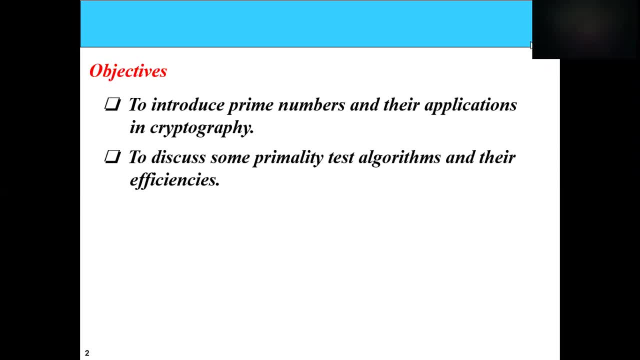 exercise the how to find out the efficiencies of any encryption, or what you call the efficiencies of time testing algorithms. it is fundamentally related with big O and big O- future notation land. it might be related with the computational complexity, and that involved time complexity as well as memory complexity. 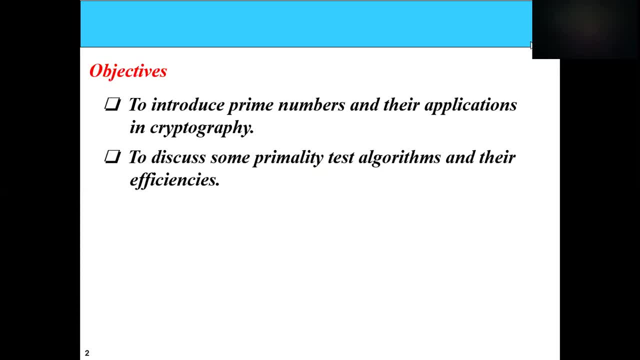 of fundamentally your algorithm. all these complex complexity theory is related with, more or less related with what you call P hard and P hard and other related, but we are not these complexity and number theoretic complexity of algorithm. so we are focus on cryptographic need of primary prime number in cryptography. so, because our 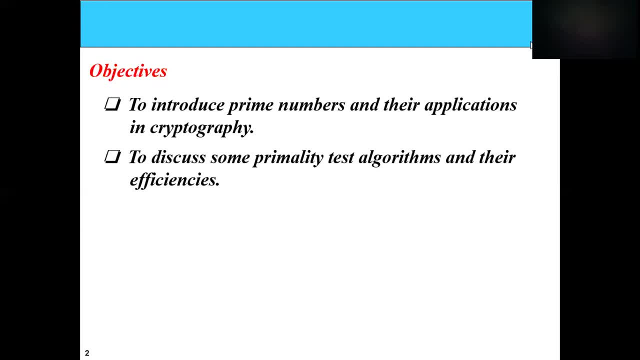 course, is related to the, what you call the cryptography, and let us today, today, the objective of our class is right this on in this slide, but which will be covered in this lecture today lecture basically related with the definition, cardinality of prime numbers, checking for primeness, then some number theory theorem, like Euler phi theorem. 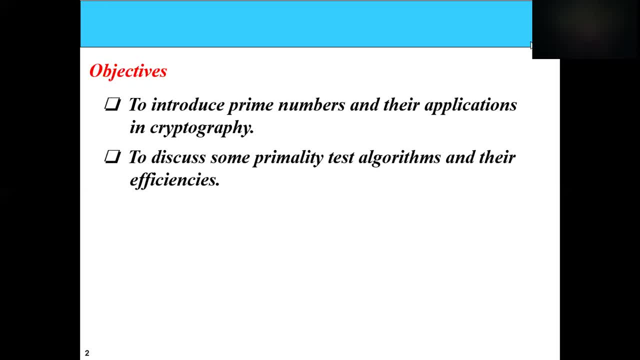 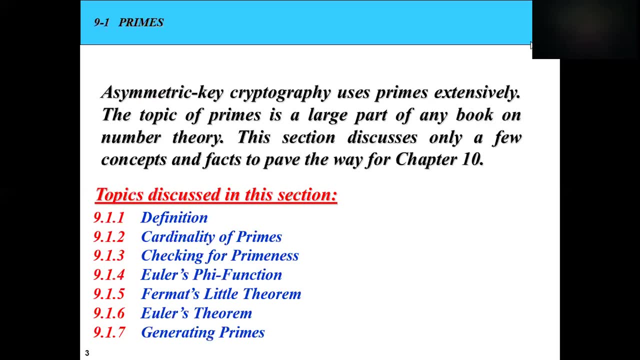 for my little theorem, either theorem and then how to generate prime numbers. so, dear student, let us start with. these are some topics, and I just take these definition for chapter 10 or 9 or 10 of what you call the book of. let me give you either the cryptograph in network security by DrinkCannabis. 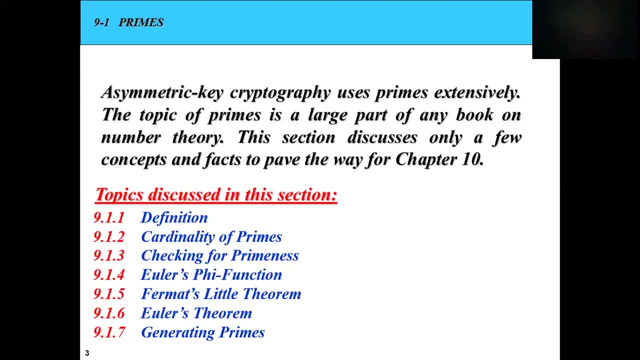 first edition Barros, frozen, and then another chapter, fundamental of cryptographic characteristics or Boolean function, a review by dr fatal automobile and Dr Matica and then introduction, the information security system. your paragraph 2.3 could be coming that information security system 2.3 and 2.6, multi of the data set Soeste. 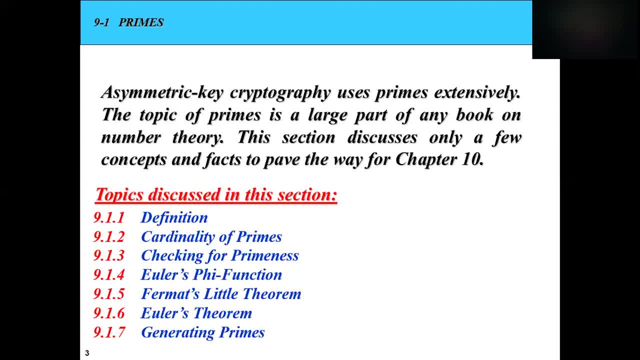 cryptography and information security approaches for images and videos. book chapter taylor and francis. these references are given at the end of uh this uh today lecture. so, uh, let us start with so to uh topic of discussion in this section: the definition, cardinality of prime numbers checking. 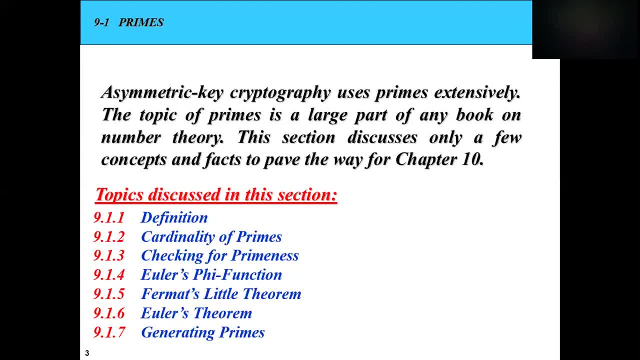 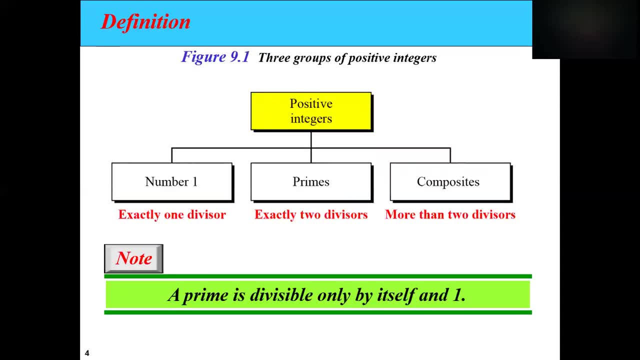 for primes, uh, eiler phi function for monitor theorem, either theorem and then genetic problems. uh, let us, uh, dear student, come up with three, uh, three integers which are quite useful in cryptography. that is first, one is like number one, that is exactly one device. it is only one number, pixel, and that is one. 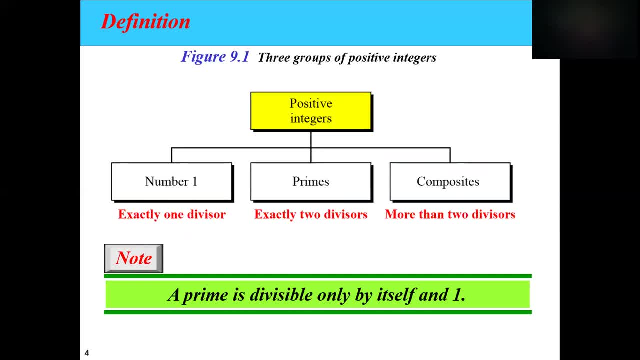 that is prime, that it has exactly two zeros, it is divisible by itself, and then unit, and unit element means to say one, then composite number. it has more than two devices. so it means composite can be baked into product of prime. what is the smallest prime number? so the smallest prime number 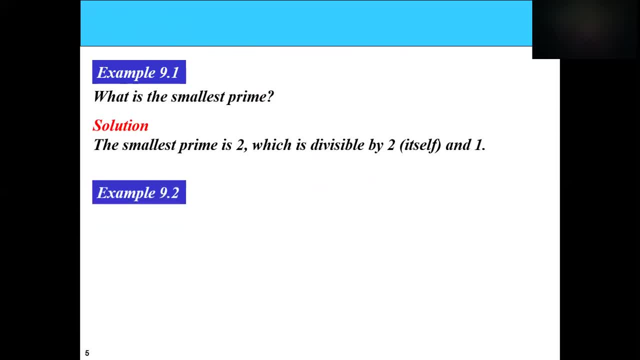 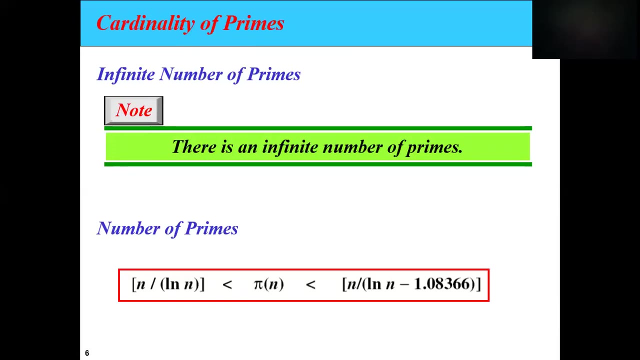 is two and it is divisible by itself and one. so, analytic term, this is the prime number. uh, less than time, that is two, three, five and seven. uh, cardinality, i need to say uh, what is the coordinate? and how many prime numbers? there are infinite many prime. 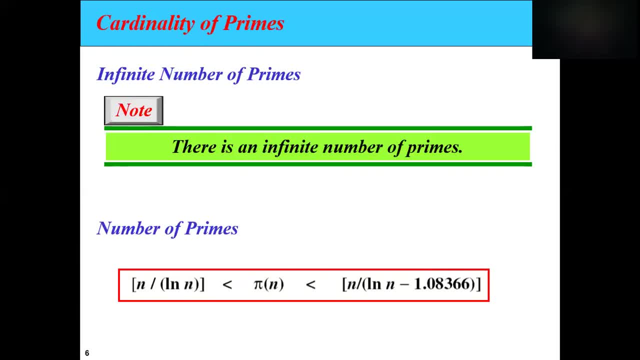 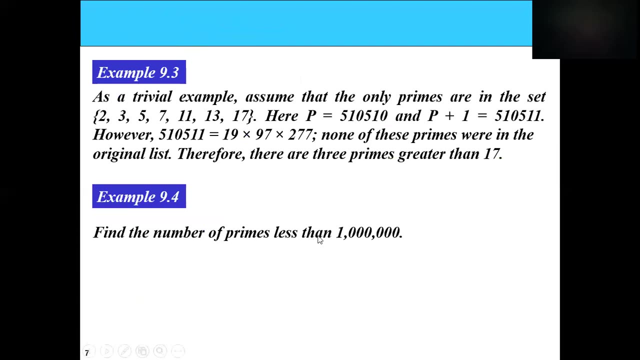 numbers. so the cardinality of prime is infinite. so the uh there is some uh lower and upper bound of uh prime numbers like this one. if i take this, find the number of prime less than uh, this uh, ten thousand, uh, how many uh uh parameters there will be? so i have to find out the uh, what you call the uh upper and lower. 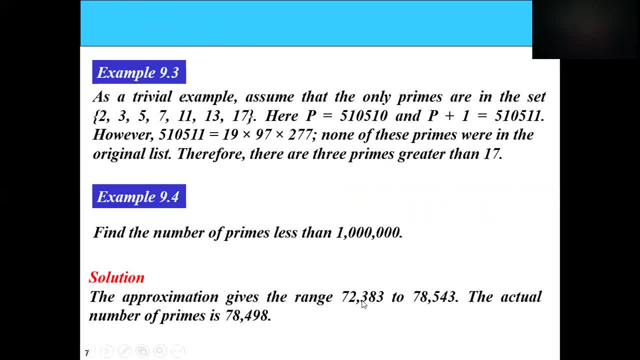 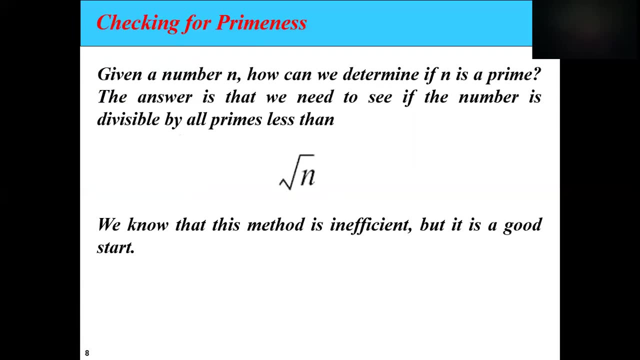 one. so the upper lower bound is 72, the thousand three hundred and eighty three, and upper bound is seventy eight thousand five hundred forty three, and the actual number of prime is seventy eight hundred ninety eight. so, uh, uh, checking for primeness, uh, given a number, and, and how can we? 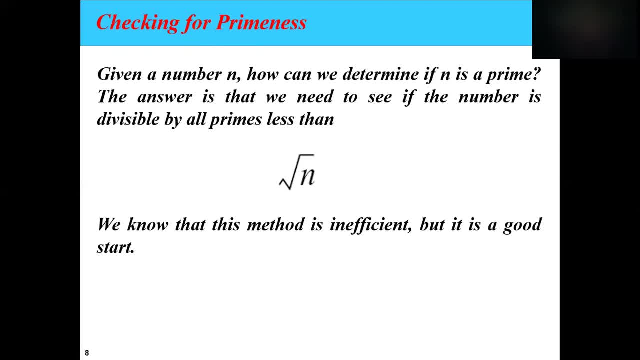 determine is it prime or not. so we have to calculate this under and uh if, after uh taking under, if you have a fraction value. so we have to omit the fraction numbers and take its uh rounded way. so, but this method is not so much efficient. but it is good for uh to start with from somewhere, so but it is again inefficient method. 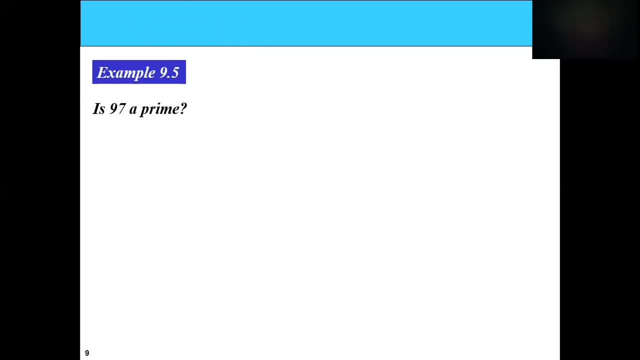 so if you can say this, one like 97 is the final mark. so i have to check, like this one i take under root of 97 and then then there will be a fraction value and that's i omit fraction, and i get nine. so the prime less than uh nine are two, three, five and seven. so we need to see if 97 is divisible by 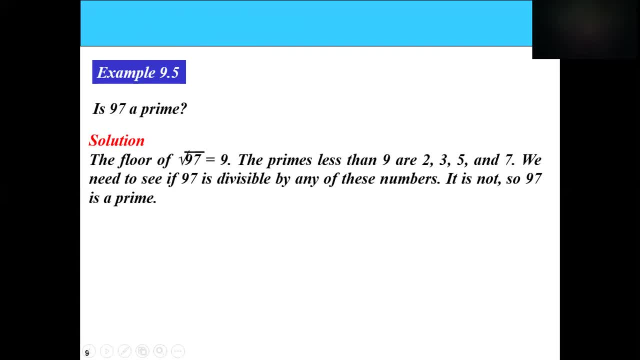 any of these numbers look so it is not. so 97 is five, so uh. first we have to take under root of nine and then we have seen the uh prime less than nine is two, three, five, seven. if uh, among these uh uh prime, if these are uh divisible by these are divisor of nine, then in that case we can say the 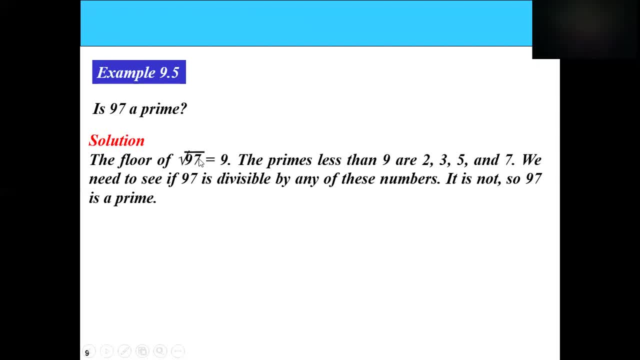 nine is uh. this is not a prime, 97 is not. if this is not divisible by uh, uh nine, then we can say the 97 is uh prime number. so in that case, if you can see 97 is divisible by uh, by any of these numbers, 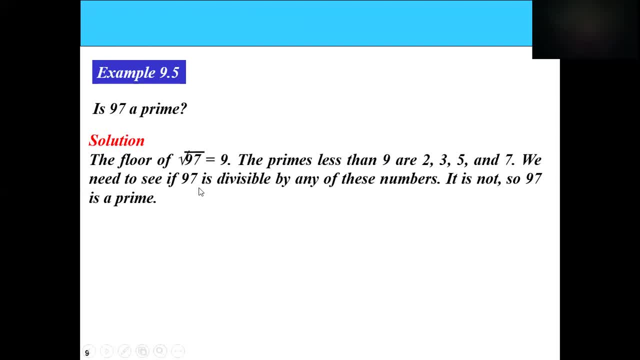 like this one uh, to see that, but it is not like this uh, from this we can say this: one, two, three, four, five num elements, uh, true, we can say these are not the uh. 97 is not divisible by 235 and 7. in that case 97 is prime. so let us take another example, and floor of 301 is 75. 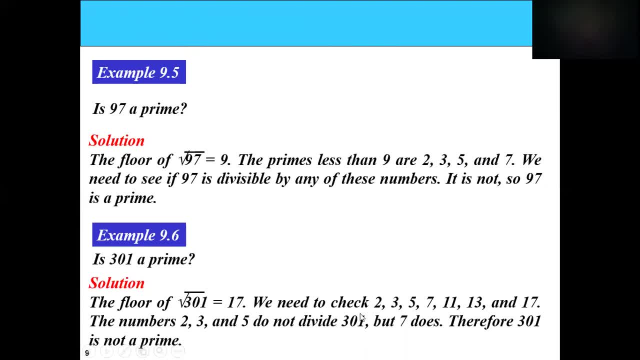 floor of 3 0, 1, 17. you need to check 2, 3, 5, 7, 11, 3 and 17. so the number 2 and 3 and 5 do not divide 3 0, 1, but 7 divide. therefore 3 0, 7 is not a prime number, so 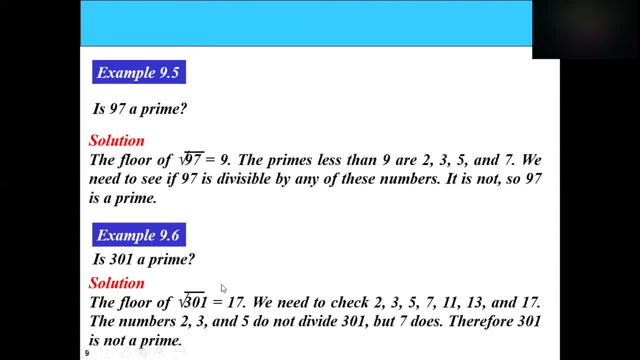 first of all you have to take the under root and then floor it. you will get 17, and then you have to find out the prime less than or equal to 17 and then you can check it out whether these time which are less than or equal to 17 are. 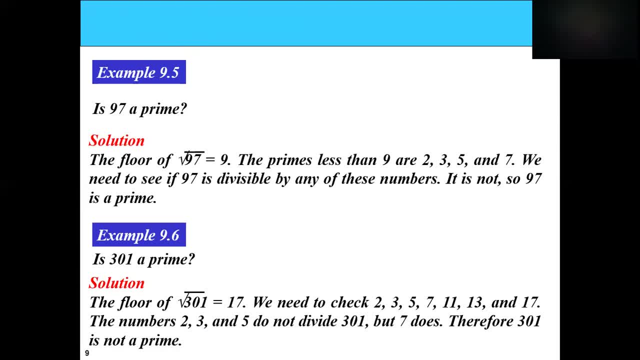 divisible by can divide 3, 0, 1 or not. if it divides, then we can say these are not in actual number is not a prime. if this is not the divide divide, then in you can see in our previous example. so in that case it is not a prime number because 7. 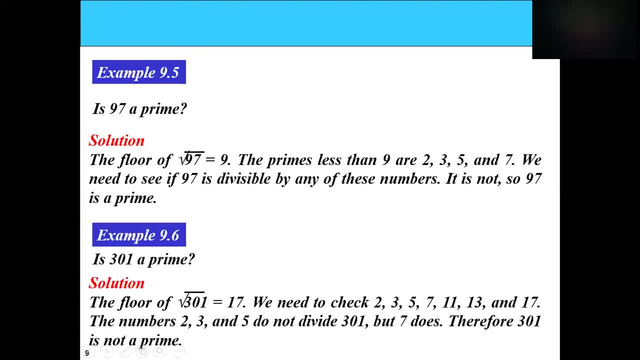 divide is a prime number. So in that case it is not a prime number because 7 divide then in, as in you can see in our previous example. so in that case it is Y is 3 0, 1. in that case we can see the student 3 0, 7 is not in time. so how many? 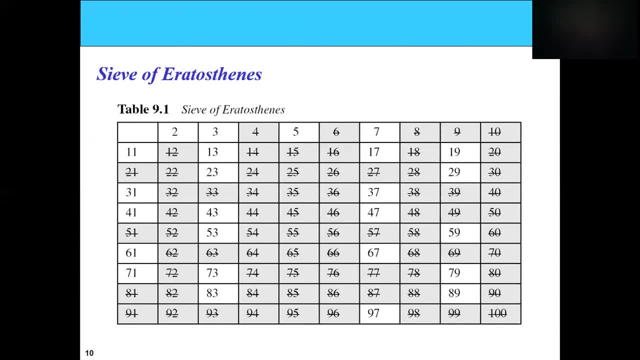 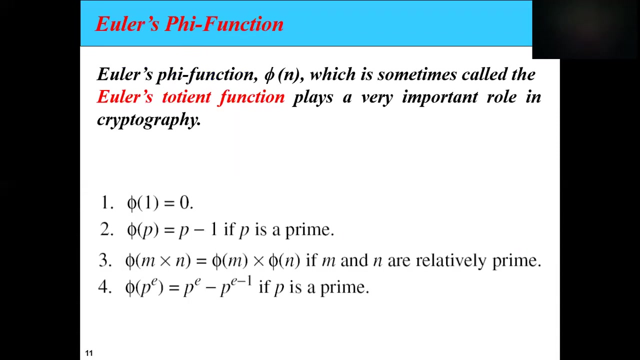 friends are existing first 100 integer. so in that case you can see over there 2, 3, 5, 7, then 11, then 13, 17, so how many are they? so there are probably 26 prime numbers in first hundred. so in that case there are six prime numbers. so I love. 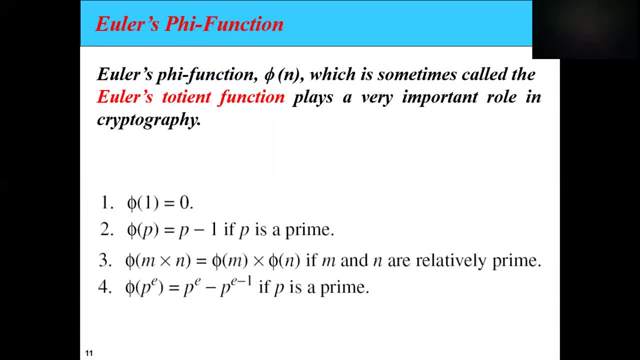 five function. I love five. function basically give you the number of unit element in any model of classes. on this player quite important role in cryptography. so I love five. function of one is zero and other five. function of P is P minus one is P is fine. I love five. 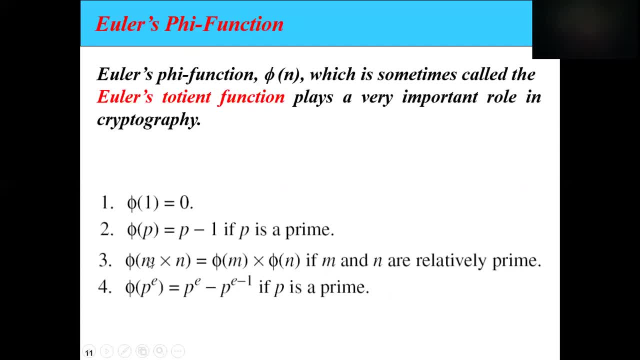 function of M cross and where M and N are relatively prime means to say their GCD is one. in that case you can take it phi of M into phi of N. if M and N, I mean so say GCD relative to prime, I mean so say this was GCD is one, phi of P power E. 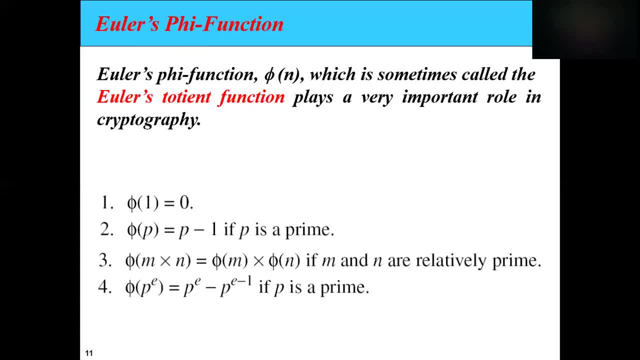 there is any integer, positive integer. so in that case the student a for this e the I love five function is a P to the power, P to the power e minus P to the e minus one. if P is fine, let us take some example. we can also: 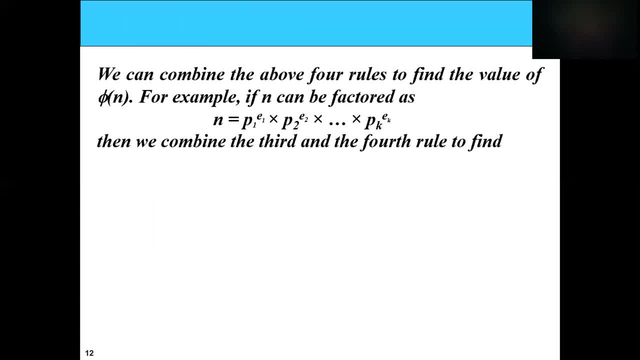 generalize these. if any number can be written as a product of power of prime, that is this one, this one, that is this one: P power, P to the power e, 1 into P to the power e. 2 into P, K to the power, e k. in that case we have found that phi of e is like this: 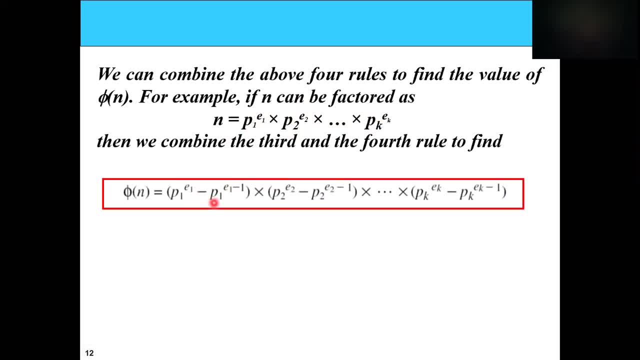 one phi of n is P 1 e 1 minus P 1 e 1 minus 1, as in our last case. fourth case: we have basically combined third and fourth case. we in that case we individually apply this and multiply the product in that case. 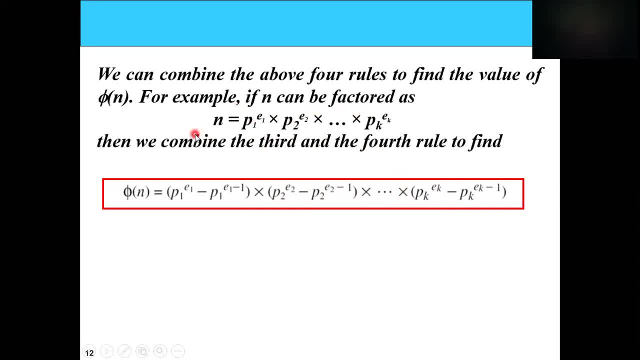 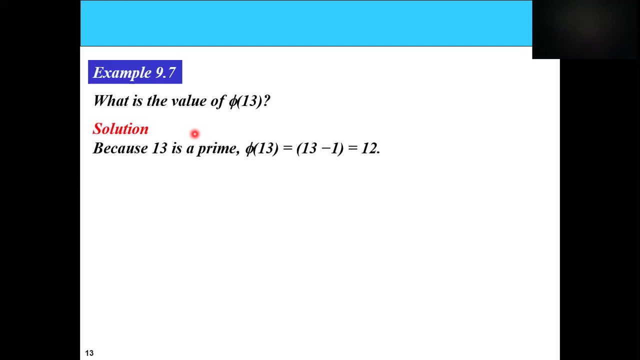 basically this is more general case as compared to last four cases. so one can say the difficulty of finding phi depend upon the difficulty of finding the factorization of N. so let us take what is the value of phi of 13? because 13 is prime in that case. 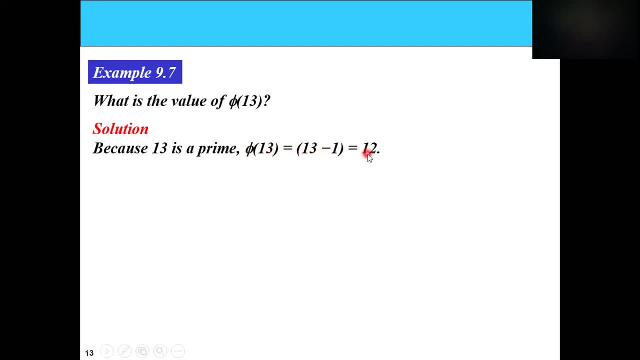 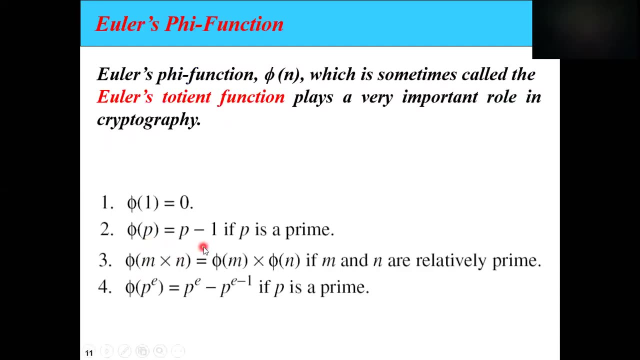 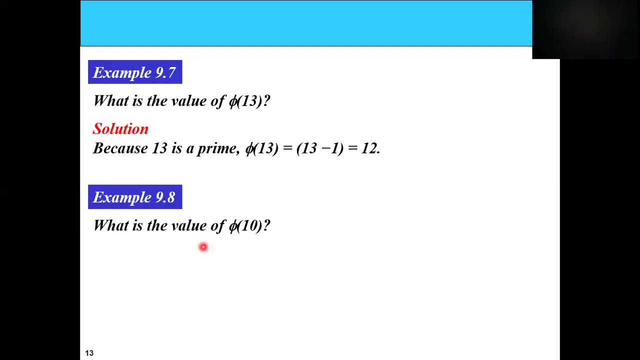 phi of 13 is P minus 1 equal to 12. we have used like this one the student. we have used this case. second case: and what is the value of phi of 10? say, 10 is not a prime and 10 can be written as a. 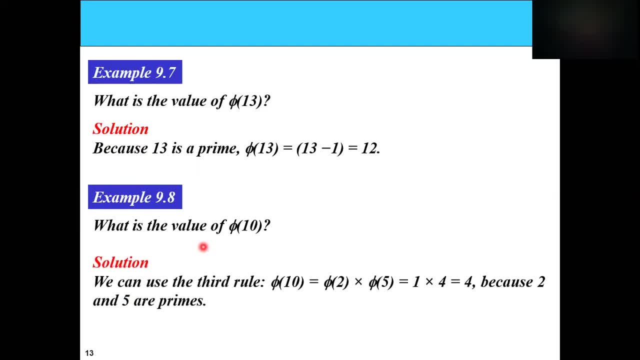 product of prime 2 into 5, in that case the student. we will use the perhaps third case which is available on slide 11. so if you can see, 2 and 3 are relatively prime. in that case, phi of 2, phi of 2, I mean. so say, since 2 is prime. 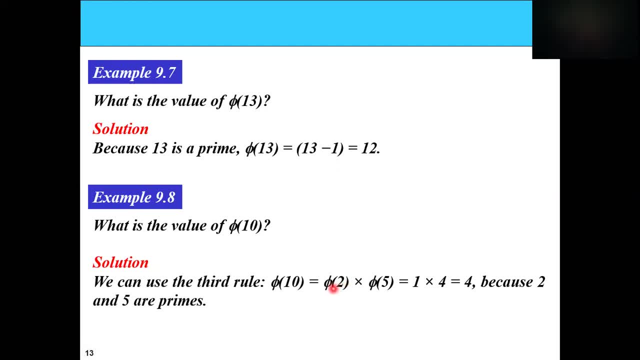 in that case we have used, that is, which is P minus 1. it means P minus 1, any. it means 2 minus 1 is 1 and 5 of 5, which is 5 minus 1, which is 4, does 1 into 4, is 4, because 2 is 2 and 3. 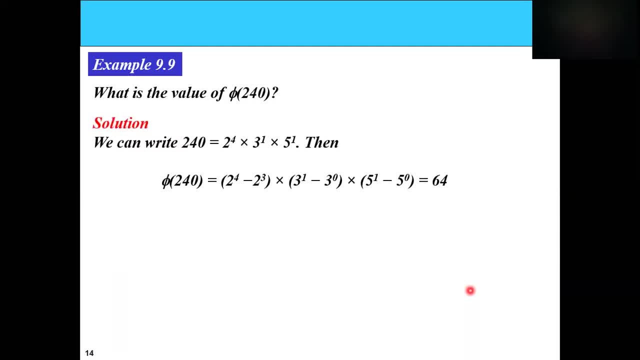 are fine. another result is 240. it can be written as a prime power product. it means 2 power 4 into 3, power 1 into 3 power 5, and in that case we will use generalized case, which is a place on slide number 12.. so in that case you can see 5 of. 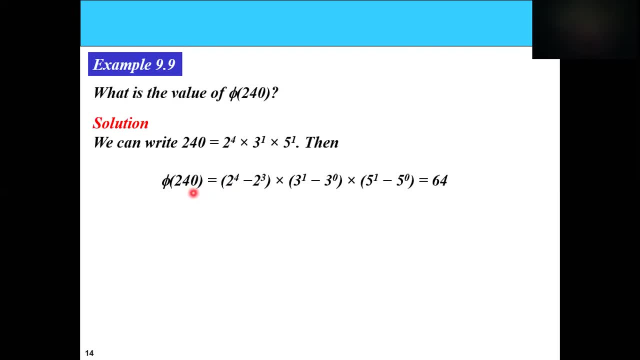 240. i means to say z 240. steric unit element in the z 240 is 64. there are 64 elements in g 240 was unit multiplicative inverse is possible. so can you say something: uh phi of uh 49? uh, it can be written as 49, can be written as a 7 into 7. 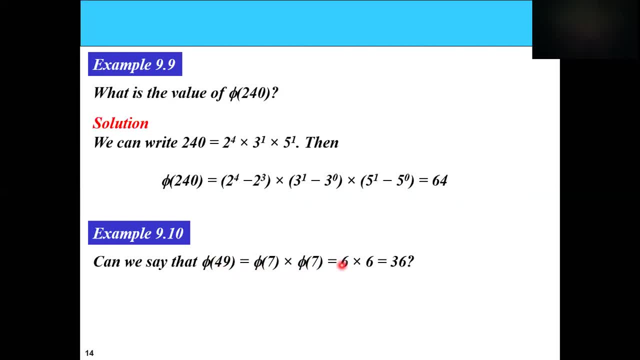 and 5 of 7 is equivalent to 6, 7 minus on 6, and then 5 of 7 is again. we use the second case of either five function uh, available on the slide number 11, but does this result is valid? no, this is not a valid result because, if you can see over here the third, 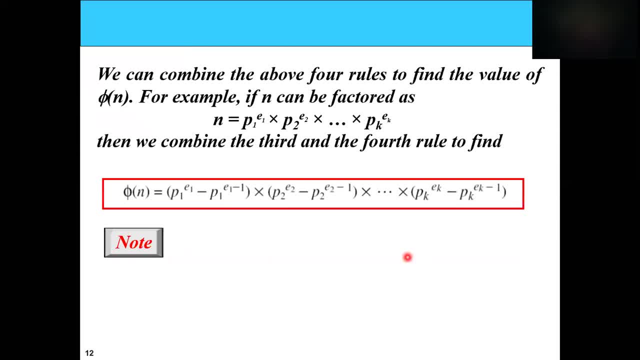 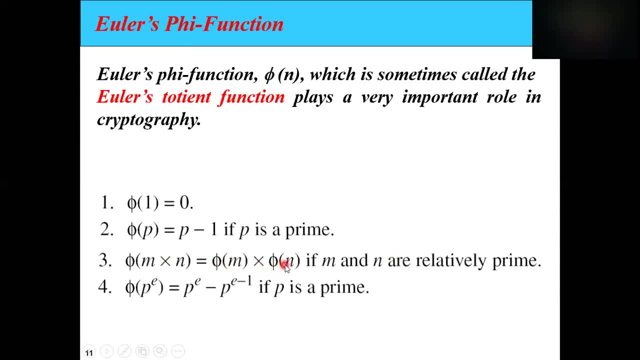 third result: uh, you can break uh and this one. this can be break if uh, m and n are relatively fine. you can see 49, 5 of 49. 5 of 49 can be written as a 5 of 7 into 7, 5 of 7 into 7, but in that case, 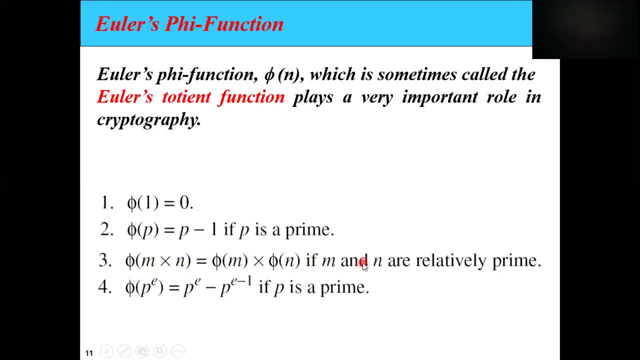 here you can see 7 into 7. the 7 and 7 are not relatively prime because the gcd of 7 and 7 is 7.. so in that case this result- you can not say the 5 of 7 into 7- can be written as a 5 of 7 into 5 or 7, because 7 and 7 are not relatively. 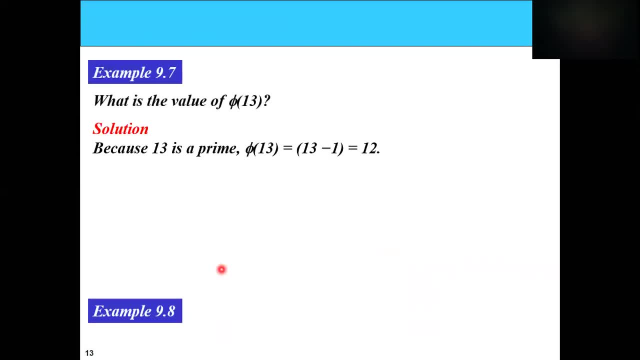 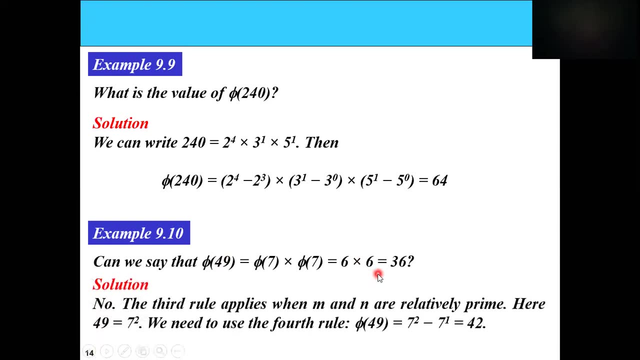 fine. so the student in that example, if you can see over here, you cannot write like this one. you can write only if these these result and this is relatively fine. so we cannot write. so we will use fourth rule that is available on slide number 11.. 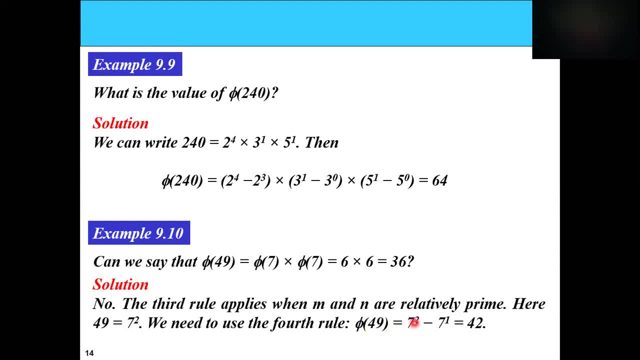 so 5 of 49 is 7 to the power 2. it means minus 7 to the power 2 minus 1. it means 49 can be written as a 7 power 2 and it means 5 of p e. here e is 2 and p is 7.. so we have used the second, fourth case. 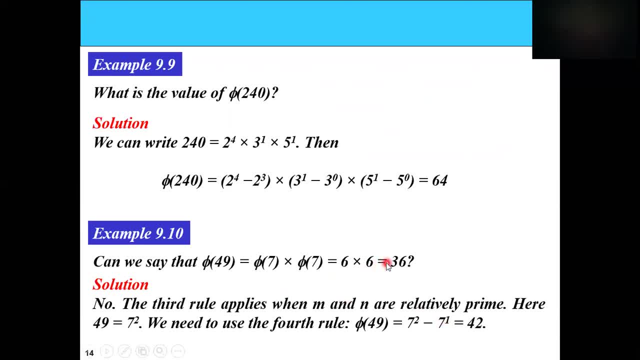 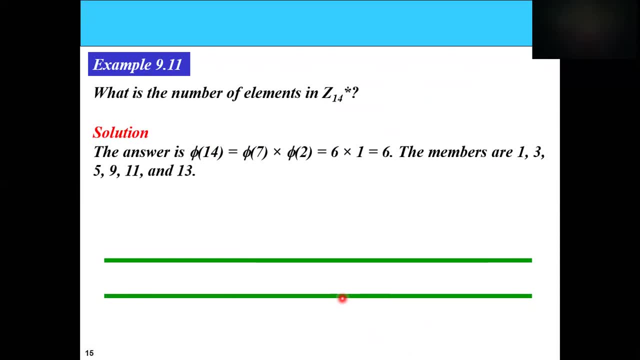 of either five function and so this is not correct so we have to use this one. what is the number of element in the z for uh four? static? i mean to say static means to the unit element. so 5 of 14. i means to say i have just read for uh 14 into a 14, into the product of 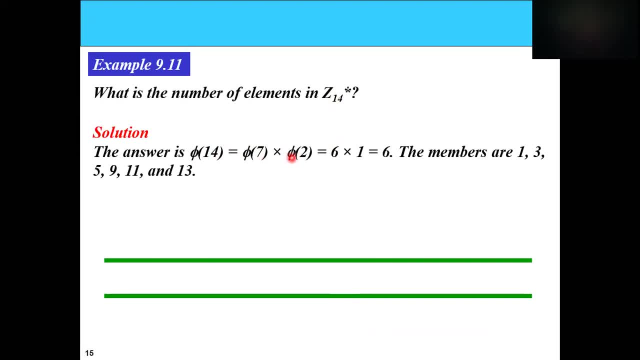 primes it is 7 into 2, so 7. 5 of 7 is p minus 1. results: that is 7 minus 1, 6, 2 minus 1, which is 1, so six. there are uh, basically unit element are in: c14 is one three. 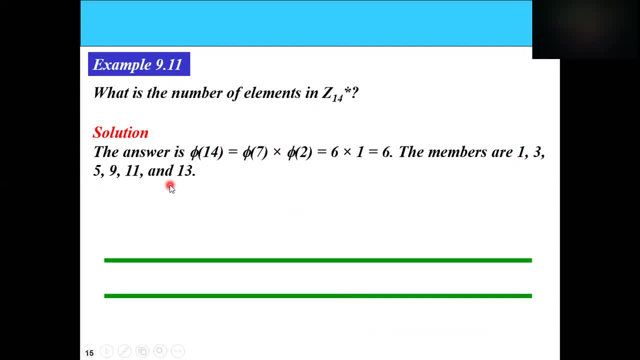 five, nine, eleven and thirteen, and also the gcd of these unit element with 14 is one. so, uh, interesting point is that if n is greater than two, then value of phi of n- this is this one, this one is- e1 is always even if n is greater. 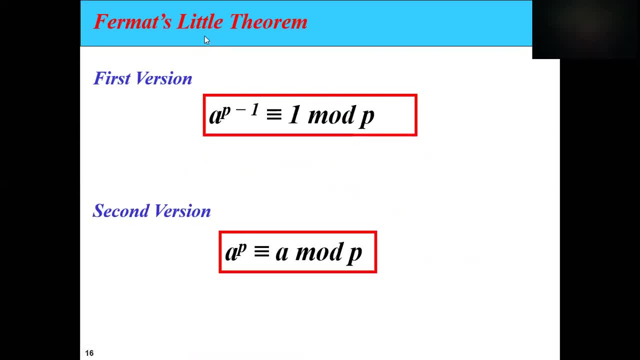 than two. so uh, their student, these are some very good in important reserve of uh format, little theorem, uh what it says: if you have any number, uh, a, and to the power p minus one is counter to one mod p. uh is first version and second one in version is: 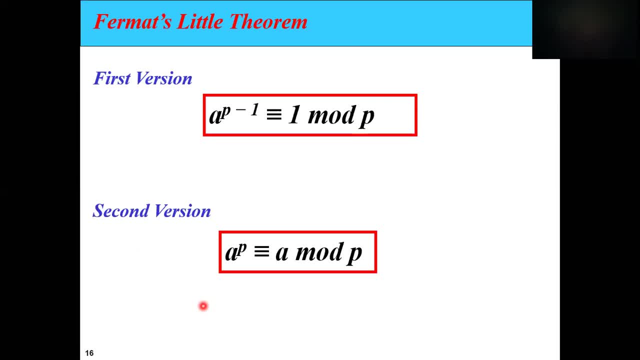 a to the power p, which, where p is a prime prime, is congruent to a mod p. these are quite important results and that is, these are very important due to the fact this is used in number of uh public key, uh cryptographic, uh the system, uh in the uh correctness proof of uh what you call. 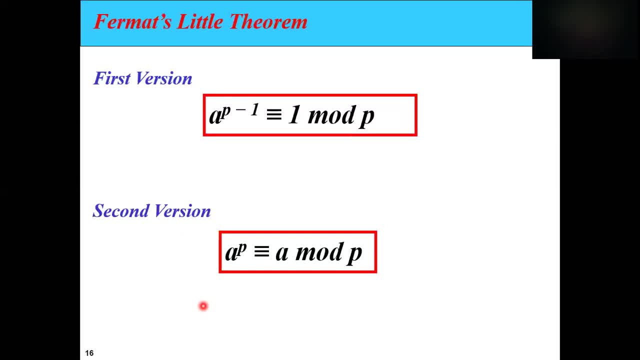 the public crypto system. so these results will be quite useful while, uh, you have, uh, what you call the, uh give the proof, correctness, proof- of your public key cryptosystem. so let us, these are some results, so you have to keep this in your mind and, moreover, these are quite useful while calculating the. 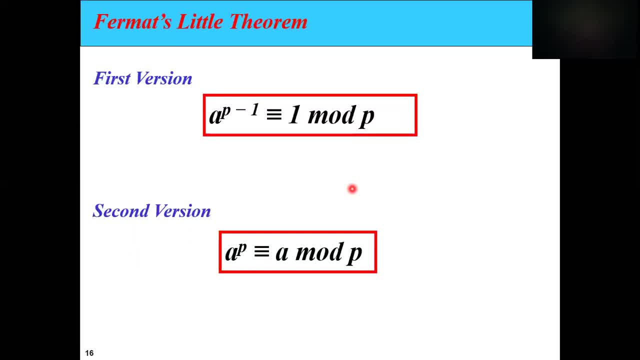 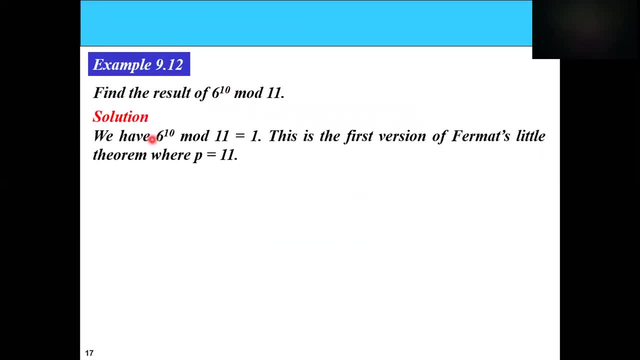 inverse in model of losses. so find the result of six and two to the power 6 mod 11.. so in that case, if you can look over here, the first fund uh version of format little theorem, that is p, is 11. so in that case, 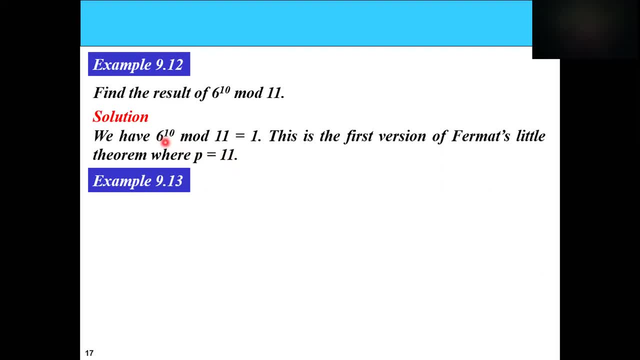 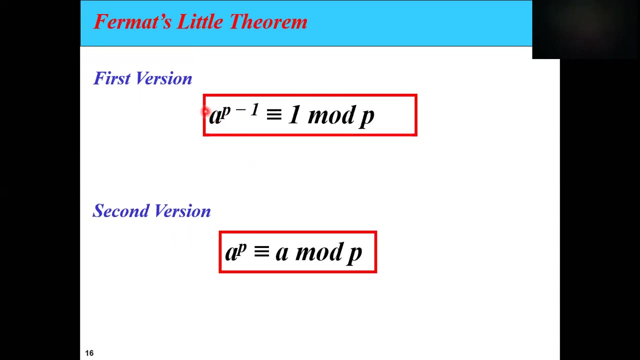 if you can look over here, 6 gct of 6 and 11 is one and this is 6 to the power. 10 mod 11 is always one because, if you can look over here, this is any element of Z P. whenever I say more P, it means I am. 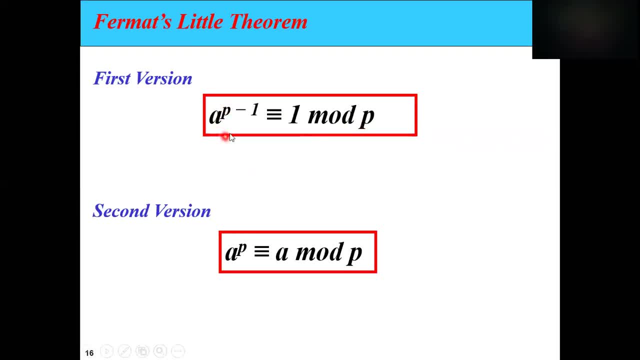 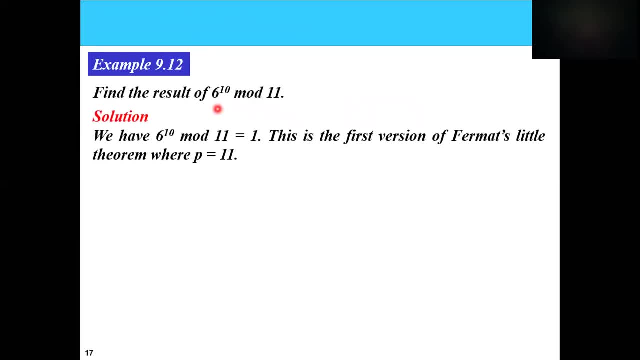 taking element from Z, P, so this is any nonzero element greater than 1. so if you can look over here, so the result of 6 to the power 10 mod 11 is 1 the more. or the result of 3 to the power 12 mod 11 is 1. so, dear student, I have to do. 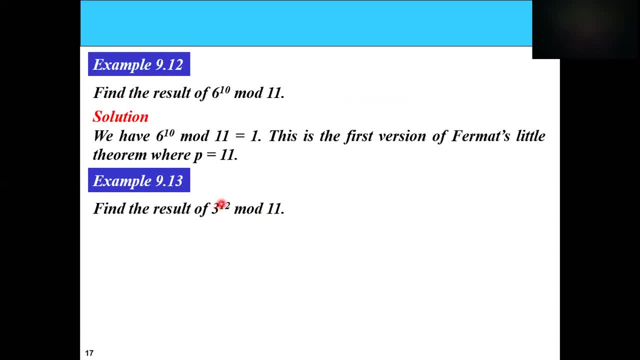 something that 3 power 10 is what you call 3- to the power 10 is 1. so I have to do is like this one here: the exponent is 12 and modulus is 11 are not same. not same with substitution. this can be solved using like this, if you can look. 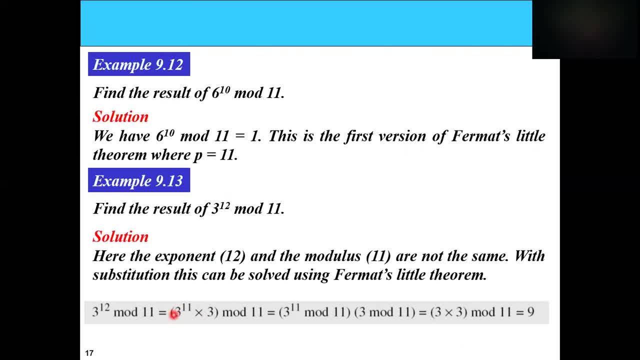 over here. so I have to break this 3 in 3 to the power 11 into 3, so 3 to the power 11 more 11 is what you call. you can see this one who have used second version of format little theorem. here we can also use the first, fundamental, first format little theorem. 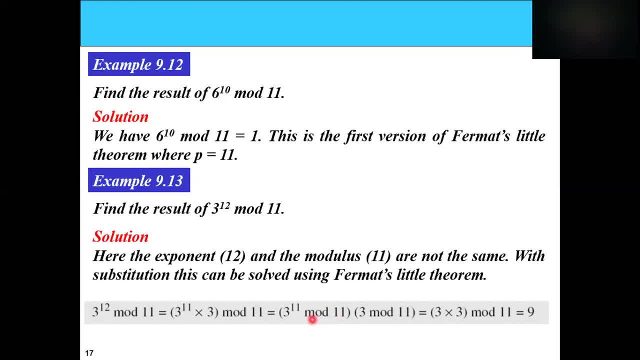 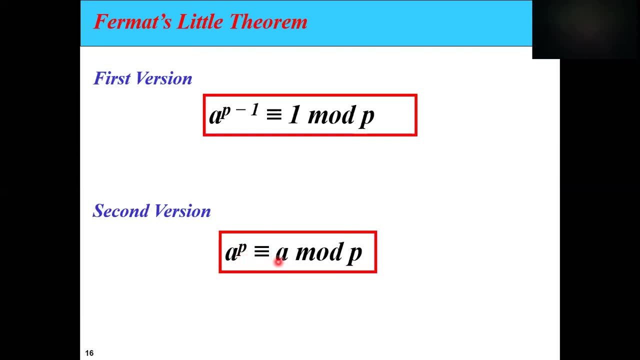 2. for that we have to use 3 to the power 10, but here we just plus by 3 to the power 11, like this one, if you can go back to last slide, like 8 to the power P, common to 8, and in that example, if you can see in that, 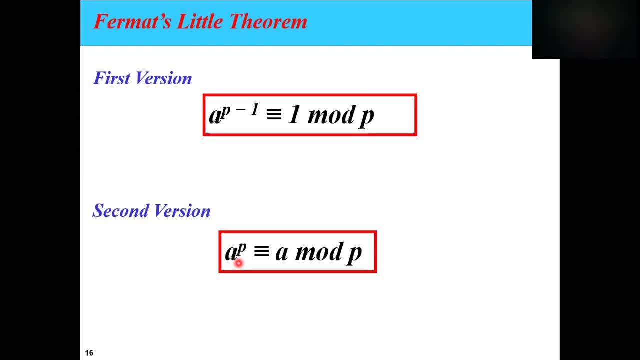 example 3 to the power 11 or 11 is give you the result 3, because 8 to the power, P is common to 8, so in that scale the student, if you can look over here- 3 to the power 11 mod 11. 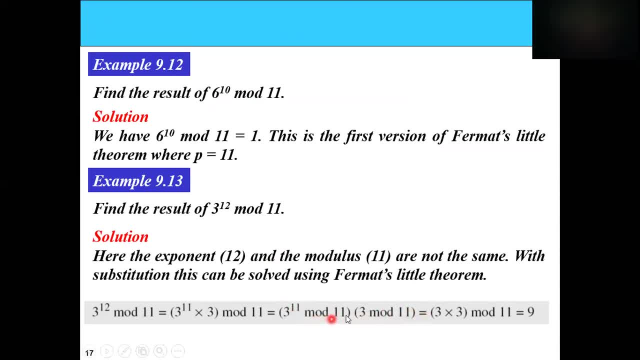 3 in mod 11. so the result of this one is 3 and the result of this one is surely 3. so 3 into 3, 9 mod 11 is always 9. so for this, if you can see over here through format little theorem, you can solve this very big power of 3 to the power 12 easy. 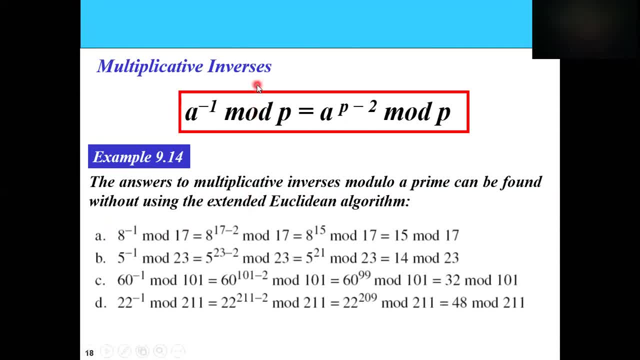 so one of the very good application of this format little theorem is to find the inverse or mod P by in last classes that we have used, including algorithm a or extended, including algorithm, in order to find the multiplicating inverses. so you can also find the multiplicating inverse. 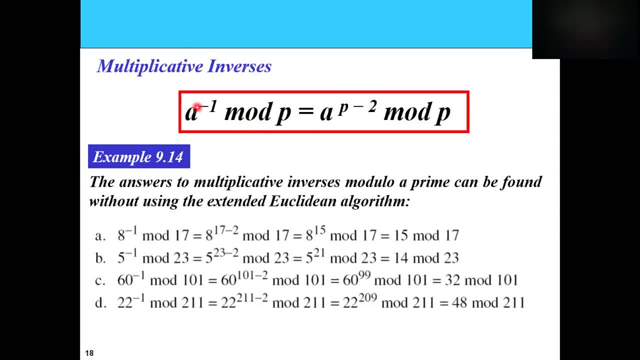 by using format, little theorem, extension of one of the extension of formality. like we have to use mod 17, so they have to use the inverse of 8, inverse of 8 mod 17. so in what? so mod 8, 17 is a to the power P minus 2, 8 to the power, 17 minus. 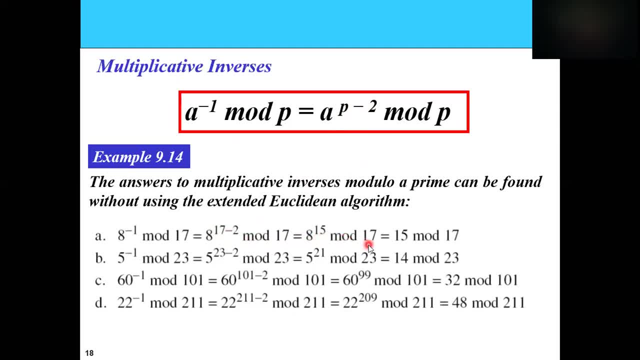 2 mod 7, so 8 to the power 15 mod 7 and 8 to the power, 8 to the power 15 mod 7 is 15, so the inverse of 8 in under modular 17 is 15, so inverse so for. 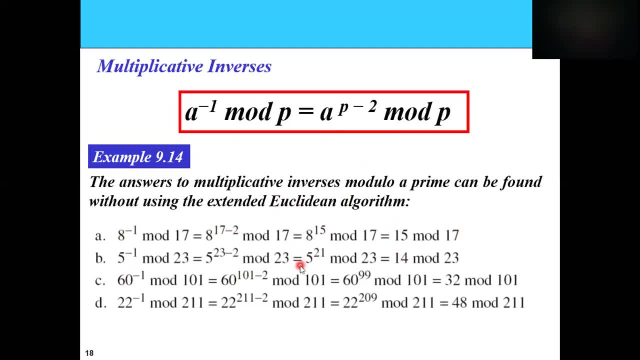 5 under mod 23 is 4, so in worst of 60. under mod 1, 0 1 is 32, so in worst of 22. under mod 2, double 1 is 40. and this is quite good manner. it can basically: 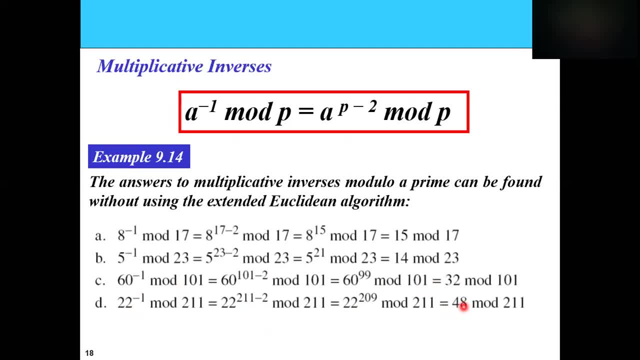 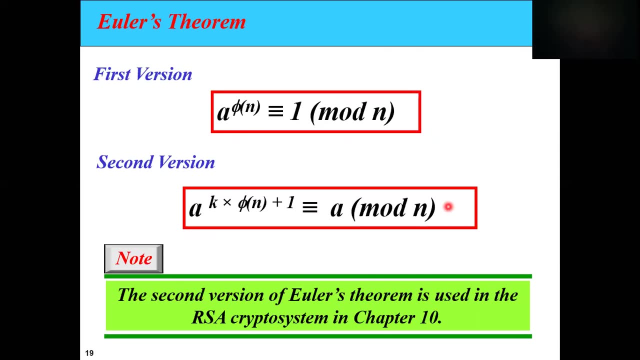 reduce your computational complexity, while looking for an effective application of this particular model, so in other words, developing it in the computer program. so you shouldn't? these are one of the application of another version, or you can say the generalization of. we call it as a Euler theorem, which is generalization of little theorem, that is, 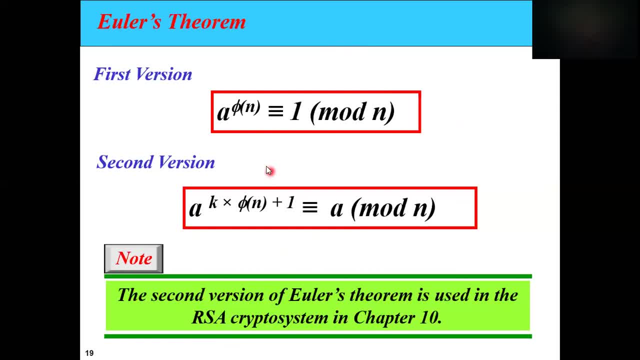 the first version of this is a to the power 5 of n is congruent to mod n and we can say this is useful for any composite number n. but the Fermat-Litter theorem is mostly useful for prime mod prime. but this is generalization. and second, 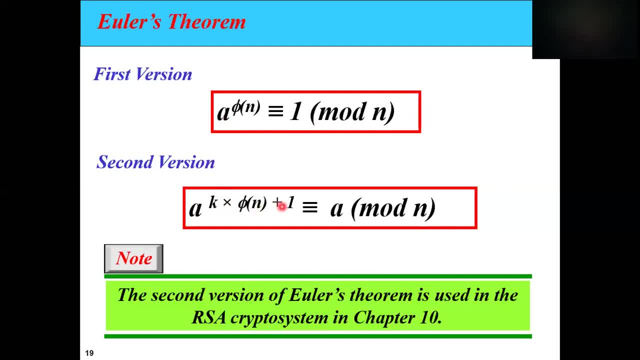 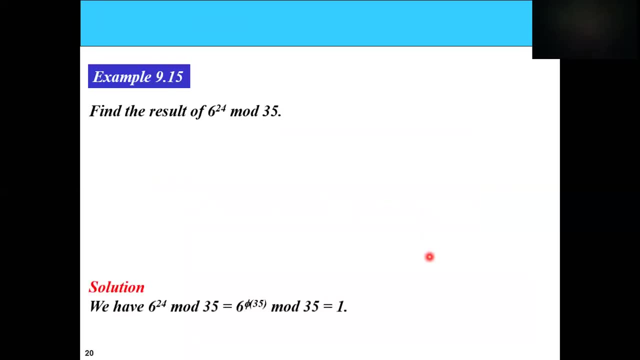 version is a to the power k into 5 of n plus 1 congruent to a mod n. so you can say: the second version of, I let you know is used in RSC, like this one, so we have any more other than prime. so in that case 6 to the power 24, mod 35 is 6 to the power 5 of 35 more 35, so 5. 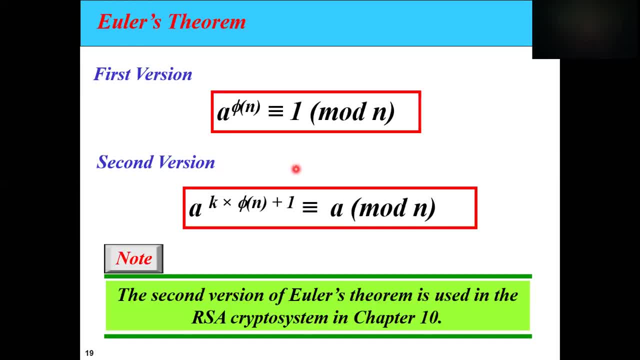 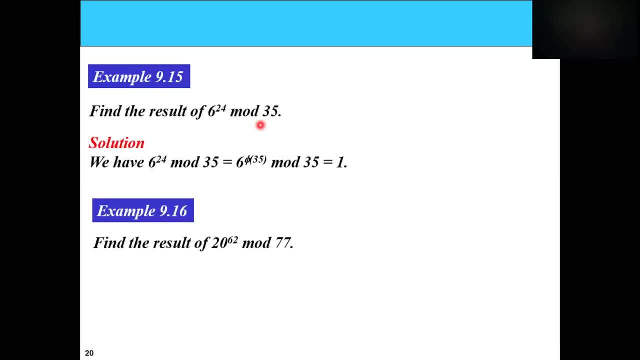 of 35 more 35 is like this. so another result: or find 6 to the 22, the power, 62, mod 77. in that case the Assurant, if you can say, take this one by of like K, is 1, 5 of 77 plus 1 and mod 77. 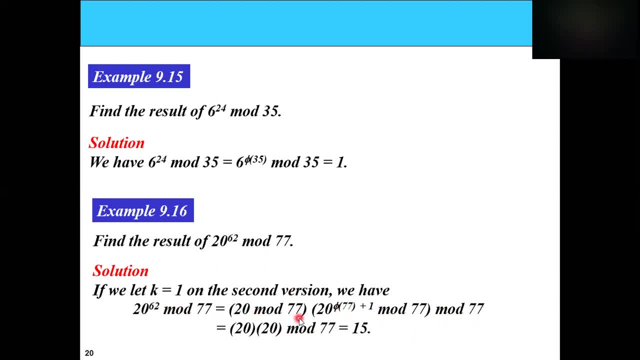 so this is k to the power 1. i means to say 20 mod 17 and 20 mod 5 of 77 plus 1. in that case our result will be 50.. if you can look over here, dear student, this will be quite easy to calculate such a big power of any. 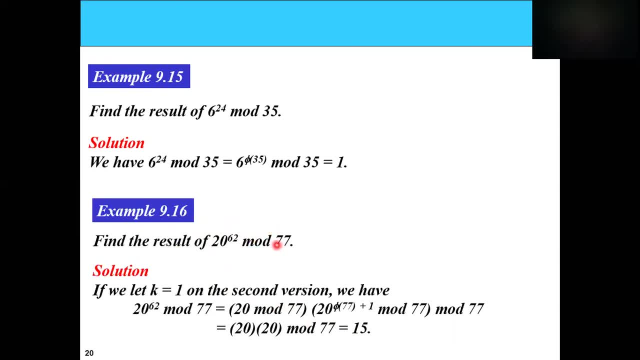 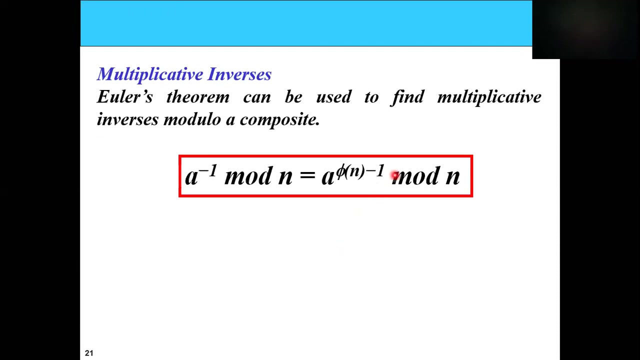 number, uh, mod, any composite number. so through this result we can easily solve by hand calculation of any modular modular operation. multiplicative inverses through mod and through this stabilization of material theorem means to the how you can use euler theorem to find the multiplicative inverse under modulo, a composite number. and 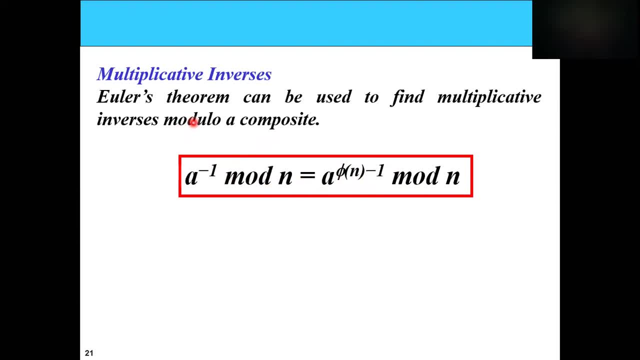 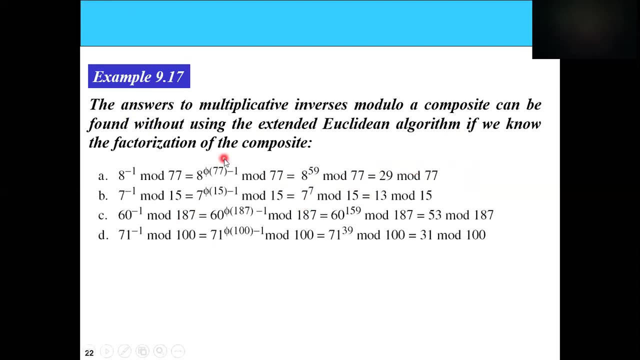 previously we have calculated the multiplicative inverse under modulo prime, but here we have used a multiplicative inverse modulo, a composite number, n. so let us take one example. so a inverse of eight more seventy, seven, seven is, uh, what you call the composite number. so five, eight of, uh, eight to the 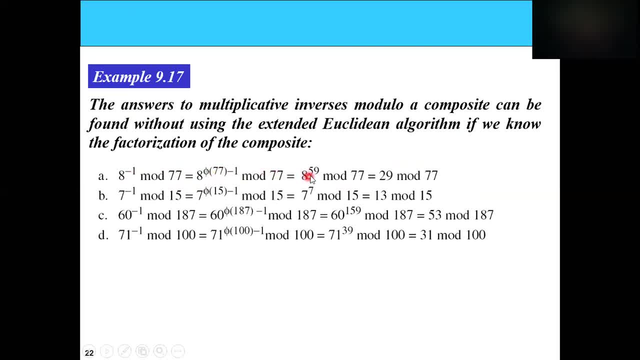 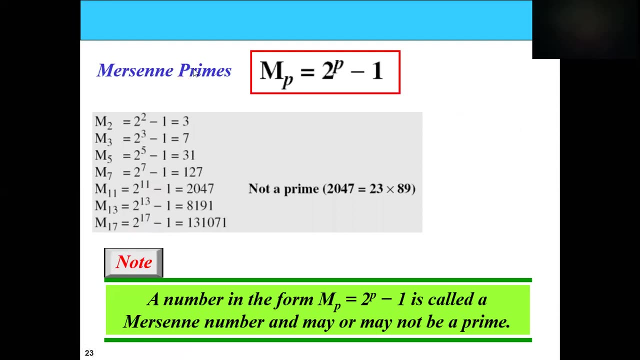 power five of seventy seven minus one mod seventy eight to the power fifty nine mod seventy, this is twenty nine. so let's the these three part. you have to do it by yourself. uh, missing, uh, prime numbers. this is another dear student. uh, one of the shortest period, if you can put two. 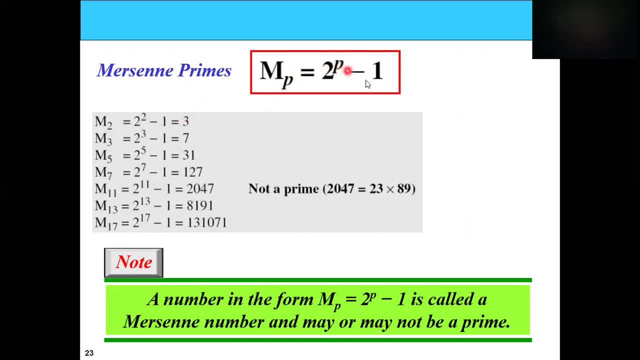 i mean two, two, two, prime, odd, three, prime two, uh, p to the power two. so if you can just put the p and the prime numbers, if you can put p is two, p, basically, p is prime to the power, p minus one. these are mercen crimes, but this is not what you call. 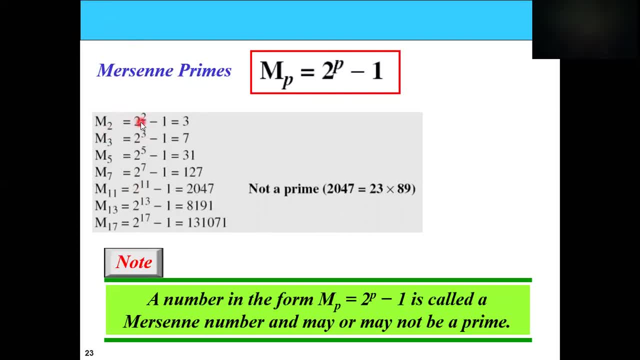 all the time. it does not, does not give you the prime. uh, it may or may not be 2 minus 1, this is 3, okay, this is fine. 3, 3 to the power, 3 minus, and this is again a prime. but for 11, the 2047, this is not a prime, because this can be. 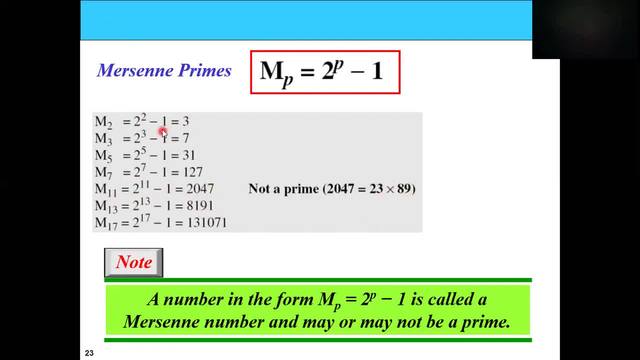 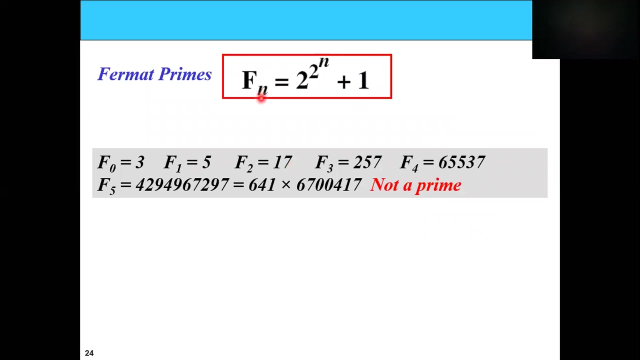 written as so. similarly, it does not always give you the prime, but it give you mostly prime number, but generally it may or may not be a prime. another result is format primes. this expression is P, F and is equal to 2 to the power, 2 to the power n plus 1. if F naught 3, F, 1, F, 2, F, 3, but for F's 5. 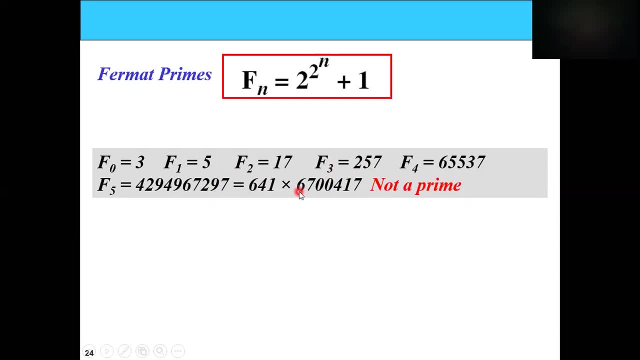 you can write it as 2 to the power, 2 to the power n plus 1, if F naught 3, F 1, F 2, F 3, but for F's 5, this is not a prime. again, the format prime is may or may not be always give. 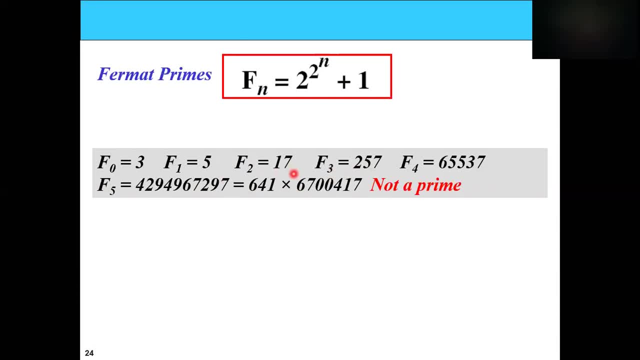 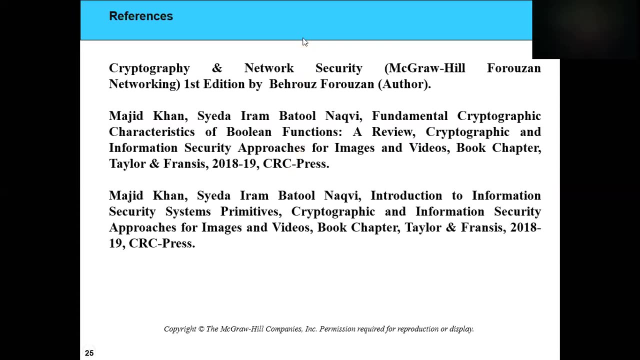